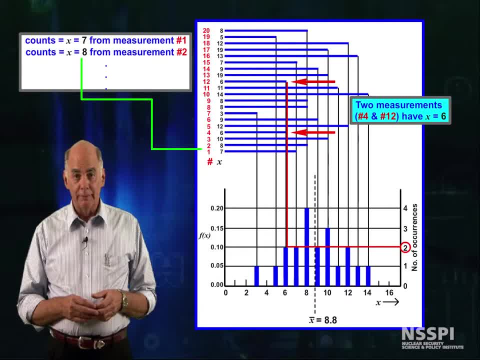 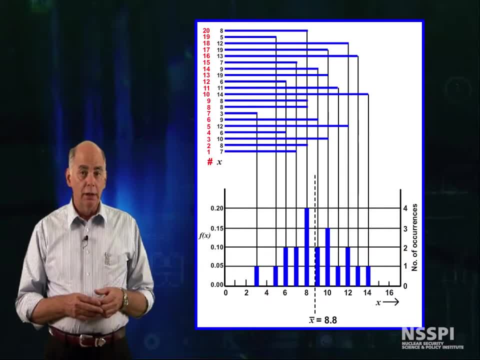 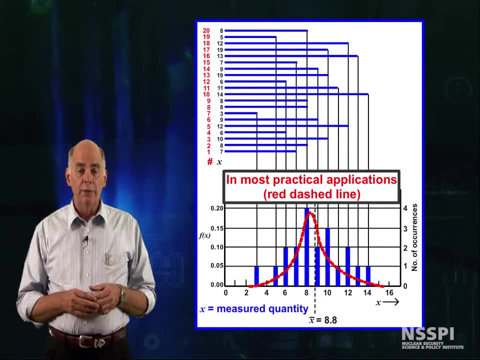 or the number of times that particular count happened. In most practical applications, and certainly for the counting applications we're going to show you in a bit the important values of x- the measured quantity, are clustered within a relative order. For example, repeated measurements of the speed of light are hopefully clustered together. 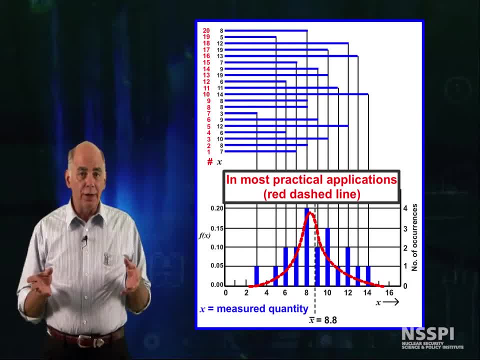 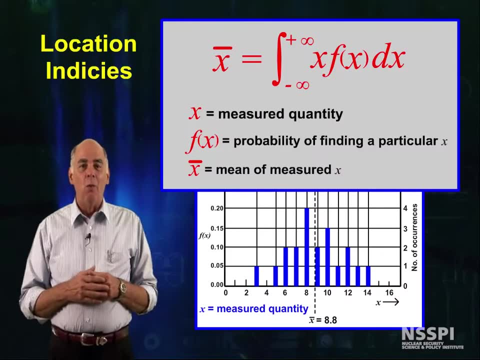 To attain a rough idea about the whole distribution of values, the position of this interval of clustered values can be described by values of x typical of this interval. Well, that sounds complicated, but it's not One of the widely used terms to describe the location. 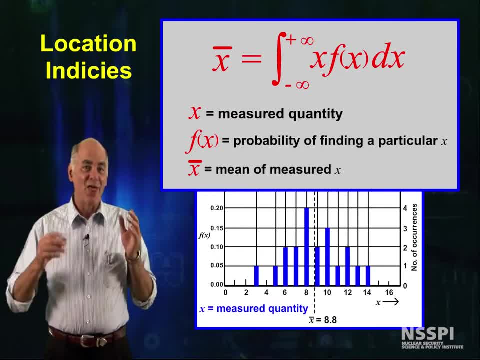 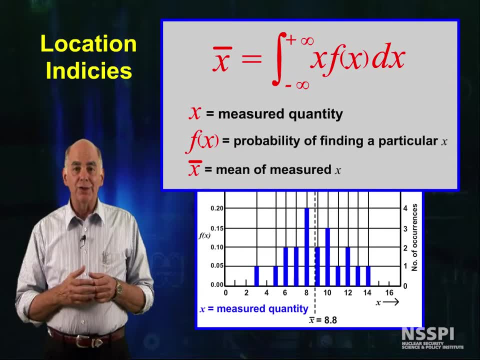 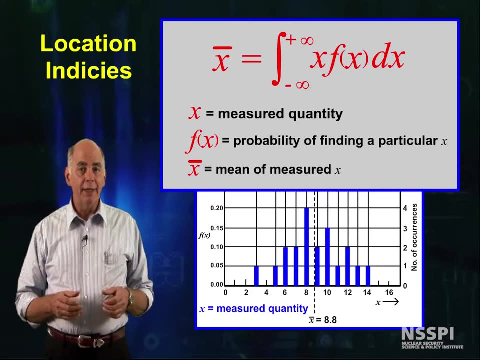 of the central cluster is the mean or the average as defined below. You probably haven't seen average defined this way, but f of x is the probability of finding a particular value of x where these x's are real numbers. X bar is the symbol we will use for the mean. 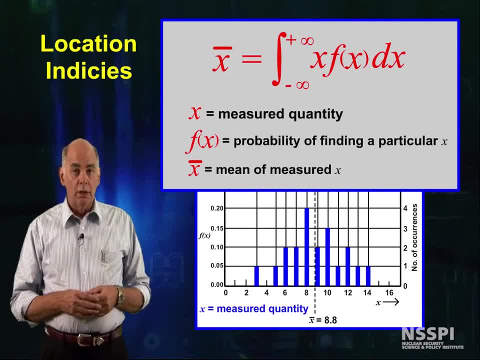 or the average for the rest of this lecture. Subtitles by the Amaraorg community. Page 1 of 2. There are other location indices besides the mean, the median, and a mode or two more that we could use. Well, it's certainly nice to know what the mean of a distribution is. 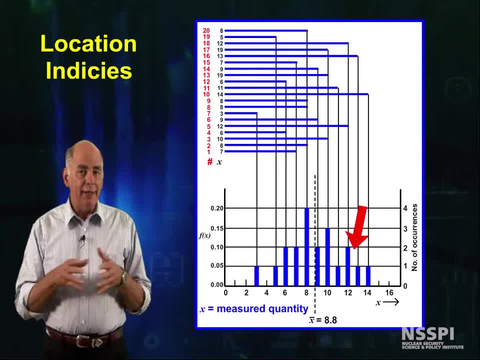 But it's also useful to know how wide is the interval that contains some portion of these clustered values. For practical purposes, it is sometimes sufficient to know the value of the location index, such as the median, or the order of the errors in the problems. 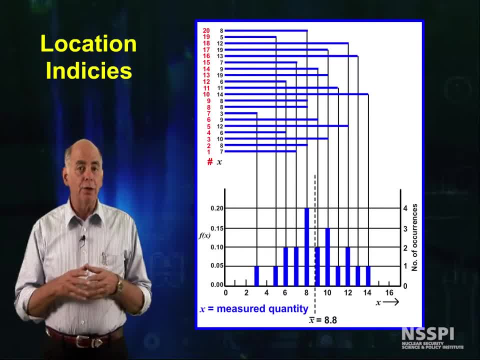 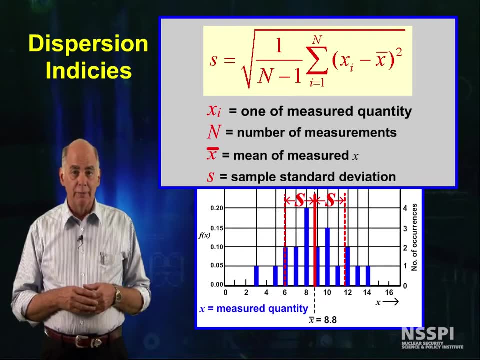 Summary of cases. Summary of cases. Summary of cases. index such as the mean and some measure of how these values are distributed around this location. index to completely describe the distribution of the variables. A widely used dispersion index is the sample standard deviation and it is defined as you see here. 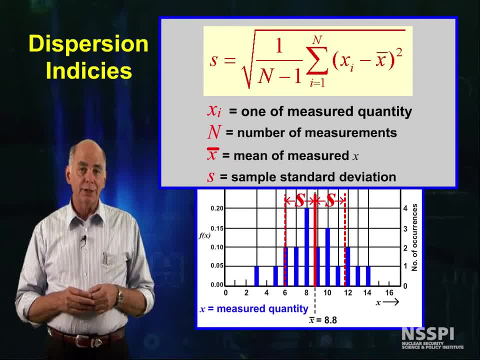 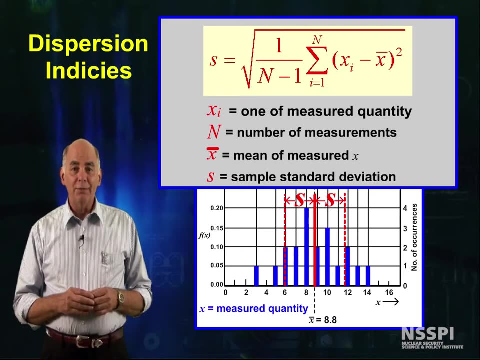 where n is the number of measurements, x sub i is one such measurement and x bar is the mean. There are several other variations of standard deviations and we're not going to get into them here. This is called the sample standard deviation. There is also a. 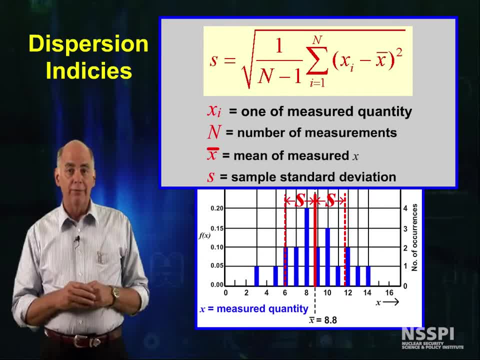 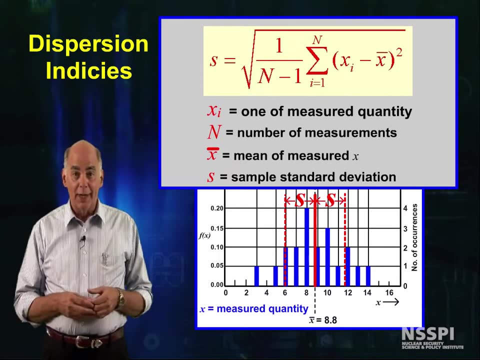 standard deviation without the word sample up front, which means you know the entire distribution rather than just taking a sample from this distribution. They are calculated essentially the same way, but the sums of the squares are divided by n rather than by n minus one. 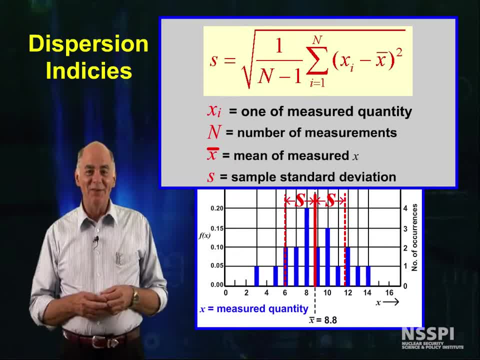 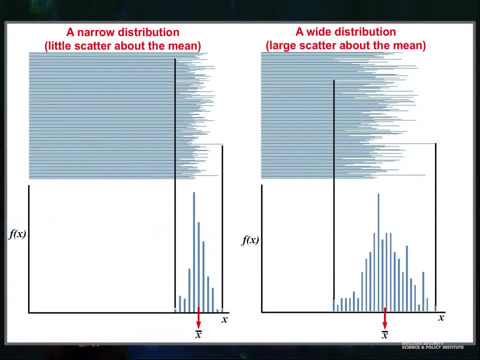 You need to take a course in statistics if you really want to understand much more than this, but that's all you'll need for this class. Here are a couple of examples to show you how standard deviations may change depending on the precision of the measurements. The 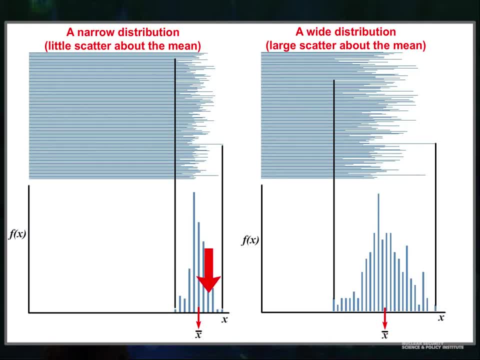 first example here has a relatively narrow distribution around the mean, so the standard deviation for this group of values is small. On the second example, the standard deviation for this group of values is small. On the third example you can see that the counts vary much more than in the first example. 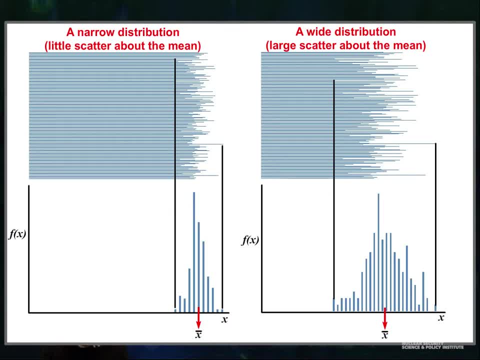 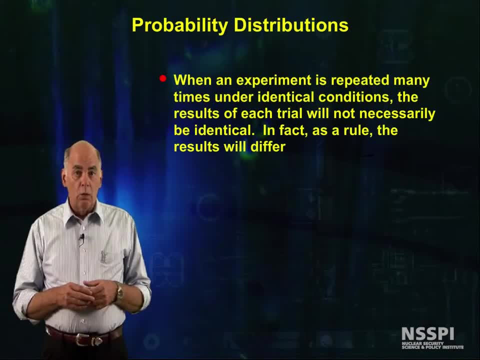 and, sure enough, the distribution varies more around this mean and thus the standard deviation is larger. To summarize, when an experiment is repeated many times under identical conditions, the results of each trial will not necessarily be identical. In fact, as a rule, the results 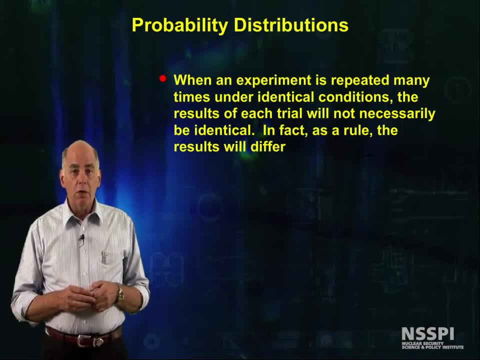 will differ. Let's take a look at an example, For example, the analysis of the mu top with a dramatic. For example, if a fair coin is tossed 100 times, the number of times heads appear will vary. If careful measurements of the speed of light are repeated, the results will differ slightly. 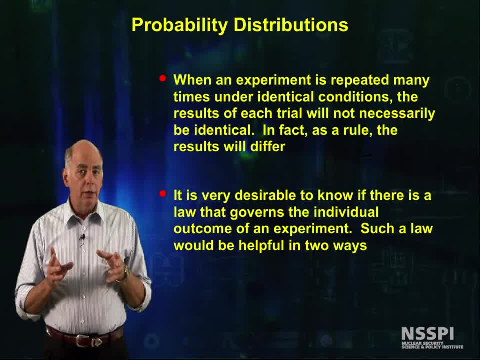 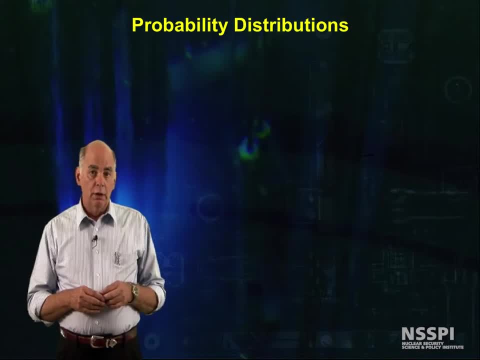 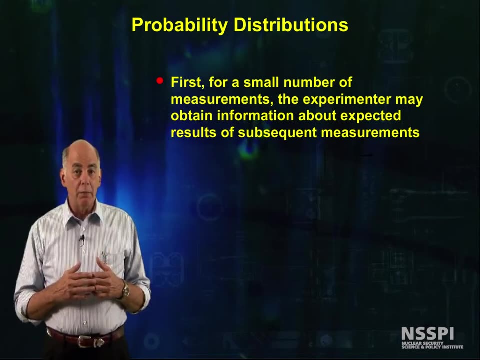 It is very desirable to know if there is a law that governs the individual outcomes of an experiment. Such a law would be useful in two ways. First, we could take a small number of measurements and the experimenter may obtain information about the expected results of subsequent measurements. 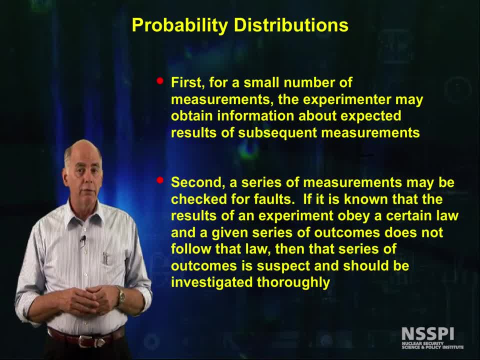 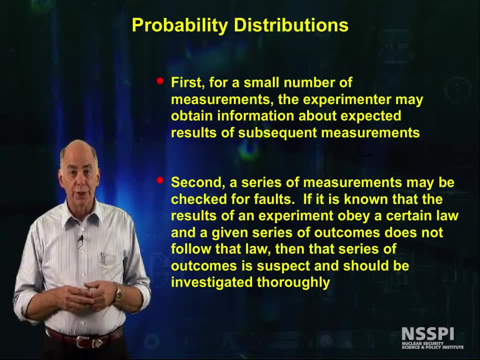 Second, a series of measurements may be checked for faults. If it is known that the results of an experiment obey a certain statistical law and a given result of measurements does not follow that law, then that series of outcomes may be wrong. That series of outcomes is suspicious and should be investigated thoroughly.